is we need to find the consecutive numbers for 63.. And what we need to do is we need to find the consecutive numbers for 63.. And what we need to do is we need to find the consecutive numbers for 63.. And what we need to do is we need to find the consecutive. 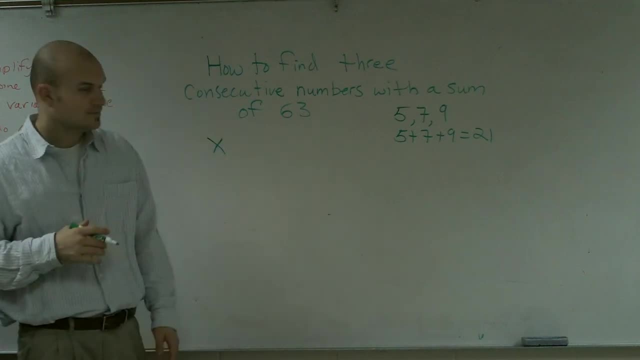 odd numbers for 1,, 4, and 8.. So to find them, we need to find a random number, from the which we leave label X. Now the next thing is I need to say: all right, well, between my next. 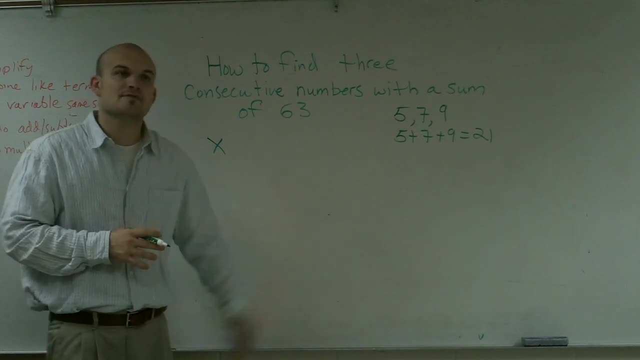 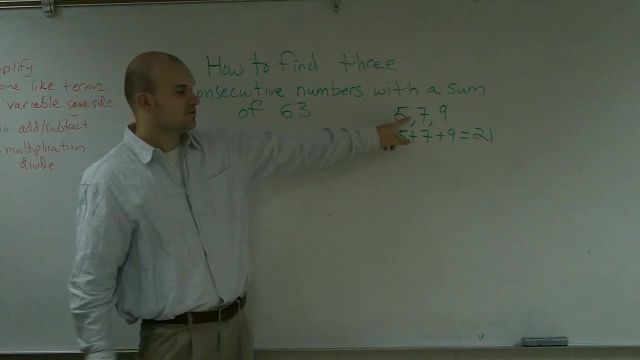 number. what is going to be my next consecutive number? Well, consecutive odd number, I'm sorry. So if I say a random odd number is X, the next one is going to be: well, not six, because six is even, it'd be seven. So it's actually you're going to have to go five plus two to get to my 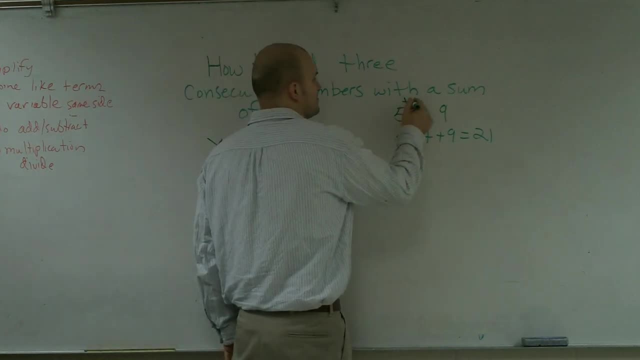 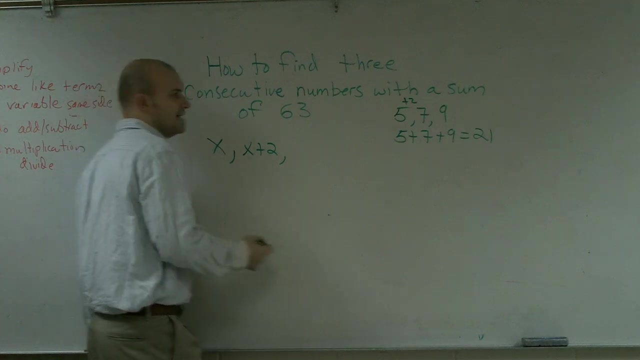 next odd number. Does that make sense? So I'm actually plussing two to get to my next number. So to represent that algebraically, I'm going to say X plus two would be my next number, And then the next number I'm going to have to plus two again. So to get from five to nine I actually 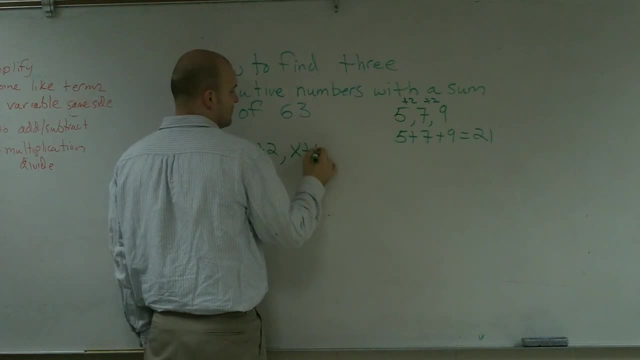 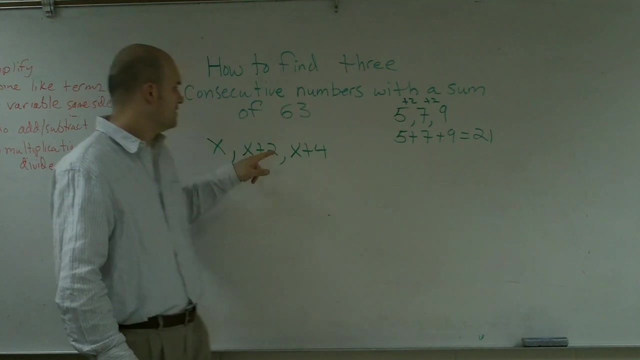 have to now plus four, So I'd have X plus four, And let's just double check to make sure this sounds correctly. So let's say X equals five. Five plus two is seven. Five plus four is nine. So this is the correct formula for three consecutive odd integers And we're talking. 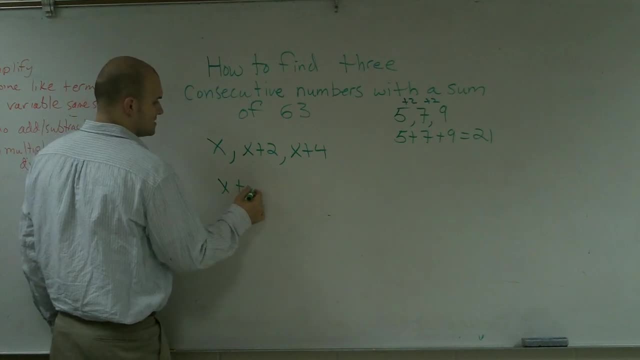 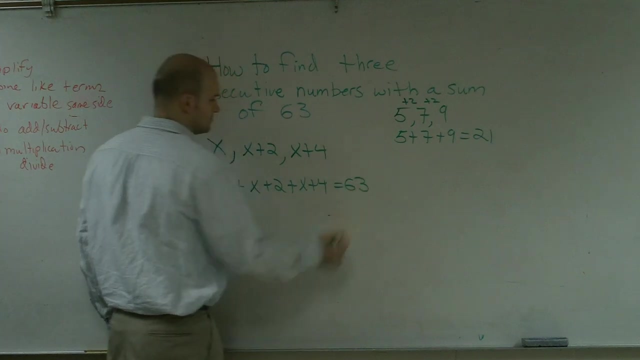 about the sum. So therefore, I'm going to write: X plus two Plus X plus two plus X plus four equals 63. Now I have three Xs on the same side. Since they're on the same side, I can combine them. So I get that three X and now I have my two numbers on. 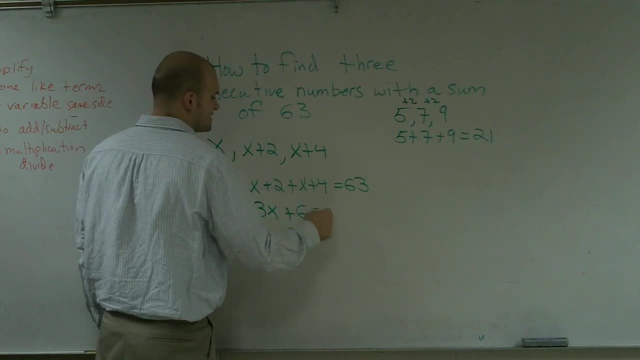 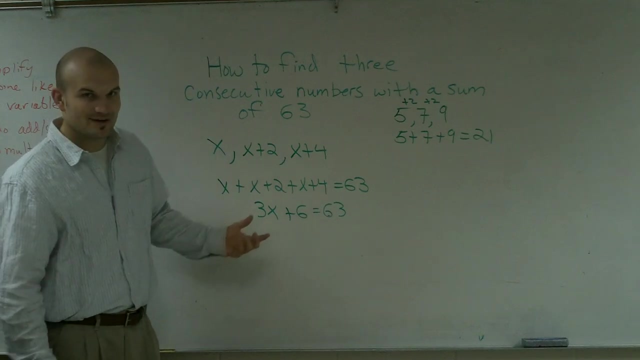 the same side. I can combine them: equals six, equals 63.. Now what we have is our lovely two-step equation, And everybody should be able to do two-step equations. If you've watched my previous videos, in your sleep you always look at your variable, you circle your variable and you say: first I'm. 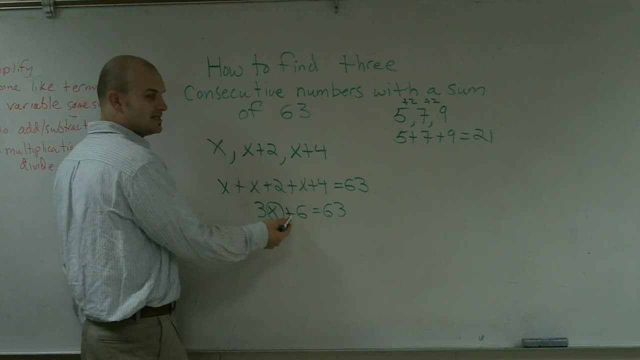 going to undo addition and subtraction by using inverse operation. Since it's being added to my variable. I'm now going to subtract six on both sides by using the subtraction property of equality. Then I have three: X equals 57.. Now I have my variable is multiplied by three, so I need